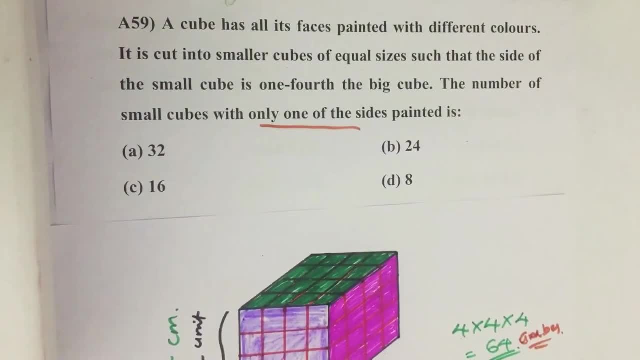 Hello everyone, here I'm going to solve 2016 CSAT question number 59 from question paper series A. A cube has all its faces painted with different colors. It is cut into smaller cubes of equal sizes, such that the side of the small cube is one fourth of the big cube. The number of small cubes 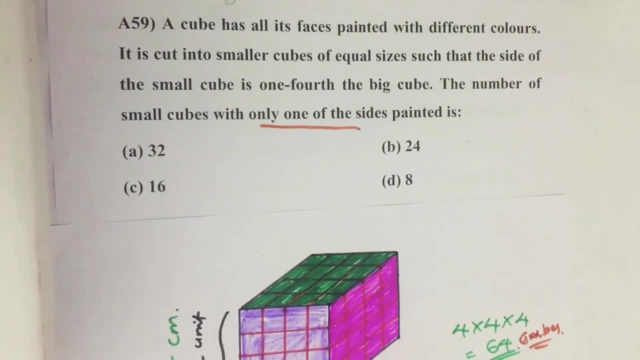 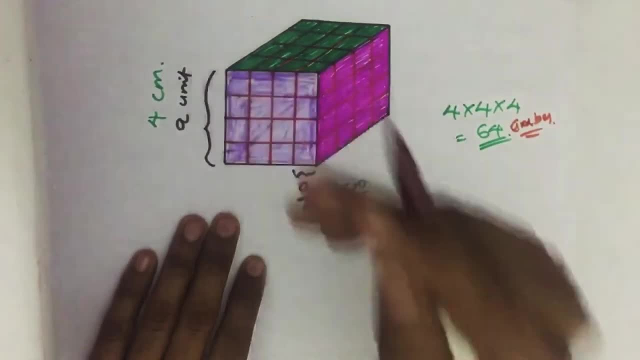 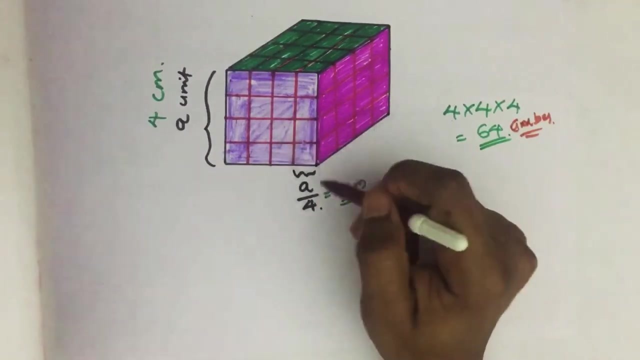 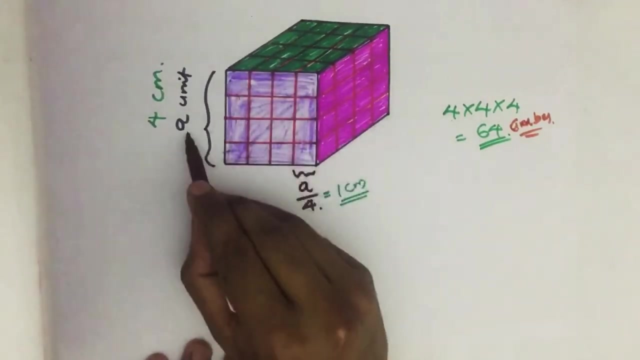 with only one of the sides painted is. So here we have a bigger cube. Consider its side equal to a unit. Then it is cut into smaller cubes such that sides of the side of the smaller cube equal to one fourth of the larger cube. This is a then side of smaller cube equal to. 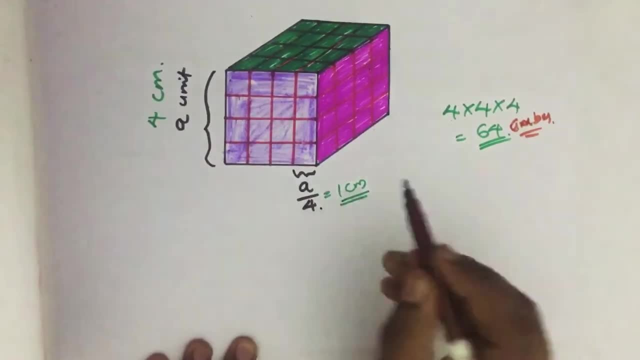 one fourth of a equal to a by four. Otherwise take one example: if side of larger cube equal to four centimeter, Then side of smaller cube equal to one fourth of four, equal to one centimeter, Then how many such cubes are possible? here it is four. 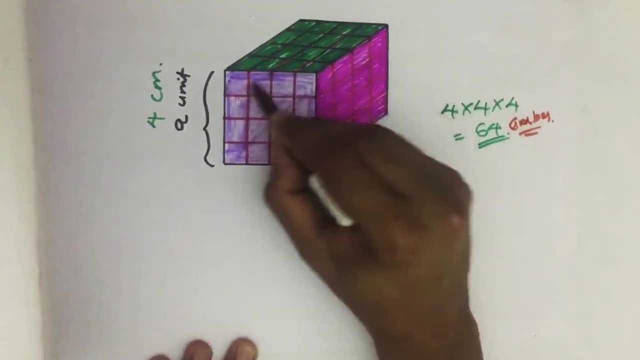 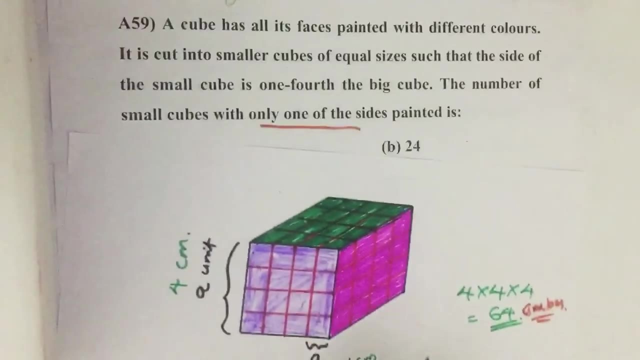 here Also four, four into 4, 16.. Sixteen. there are four such layers, Sixteen have planned it. 64 smaller cubes. Then they are asking the number of small cubes with all traits: areaney, seven, four and nine h and searched twice in the past. Are you going toιο wife? 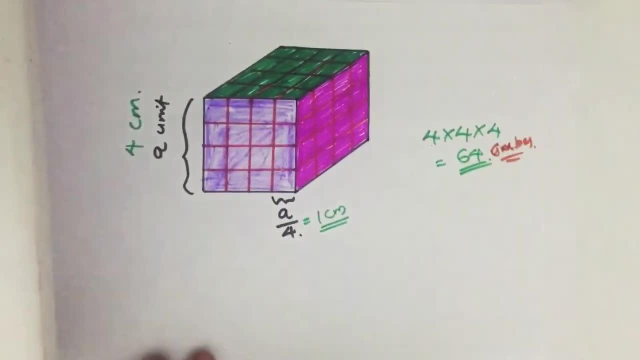 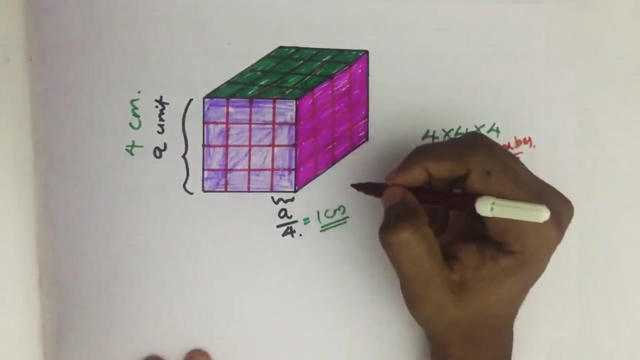 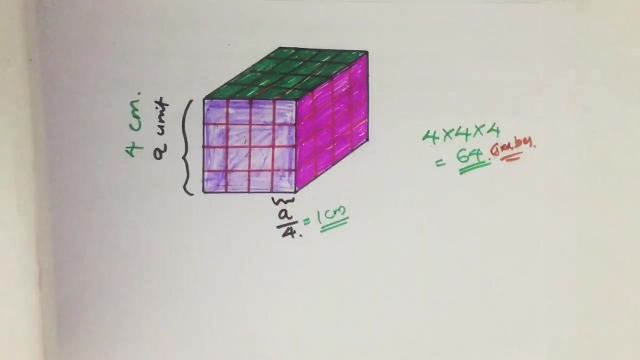 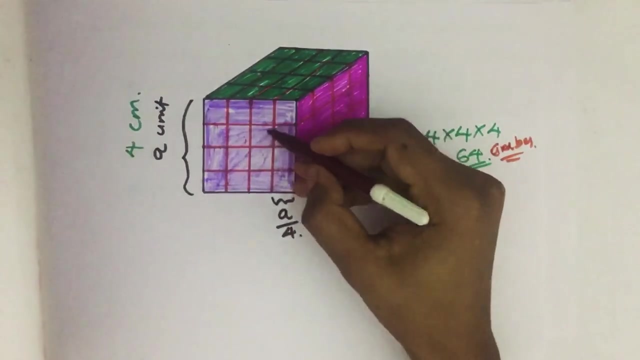 one of the sides painted is. first consider the cube in the corner. three of its faces are painted. then see the cubes in the edges: two of its faces are painted. now see the four cubes in the middle. only one of its face is painted. then there are six, face for a cube in each face. there are four cubes with only. 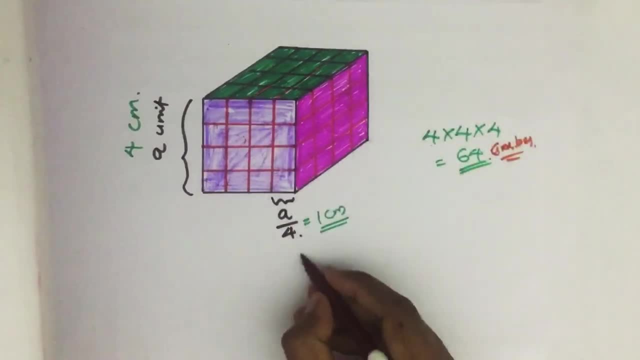 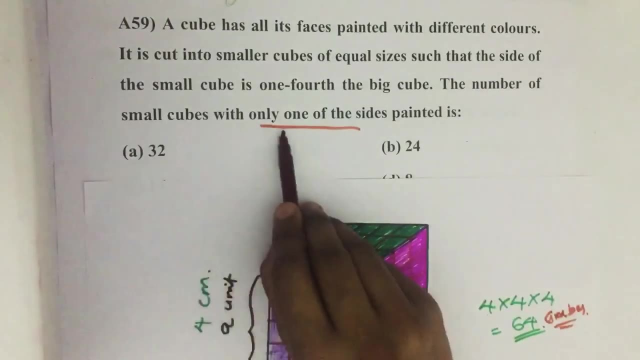 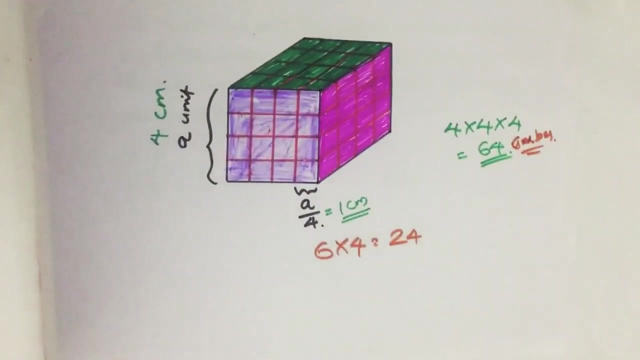 one face is painted, then six into four. twenty four smaller cubes are there with only one of the side is painted. our answer is option B 24. if you have any suggestions, please do comment. don't forget to Like, share and subscribe our channel. keep supporting and loving us, Jai Hind.